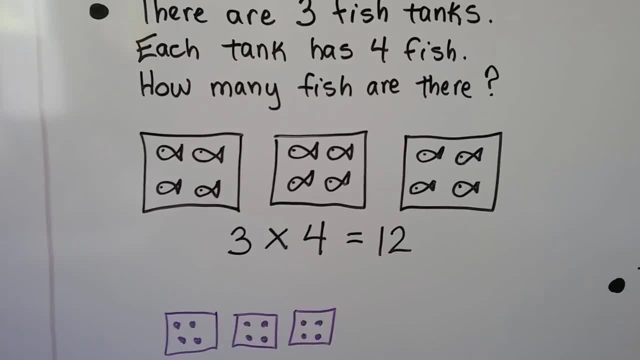 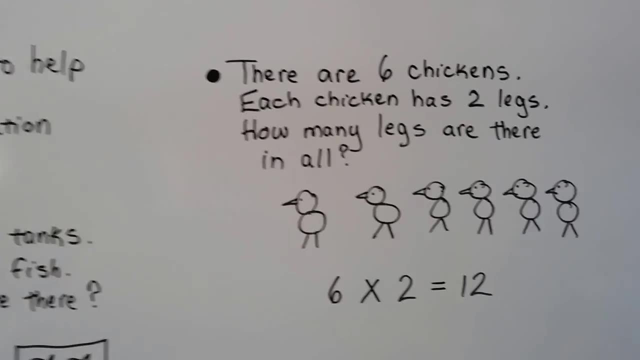 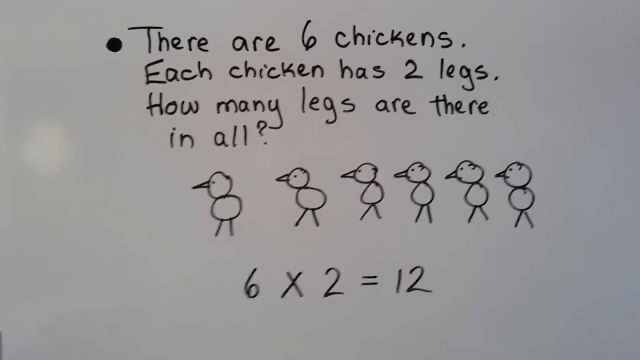 inside of them to represent the fish. Because the drawing doesn't have to be perfect, It just has to help us write the number sentence. Okay, Let's look at this one. It says there are six chickens and each chicken has two legs. How many legs are there in all? So don't laugh at my drawing of my. 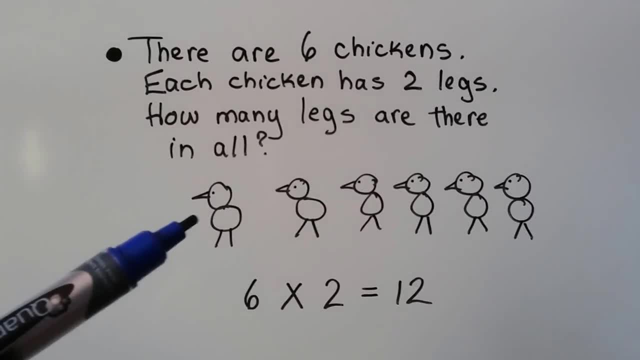 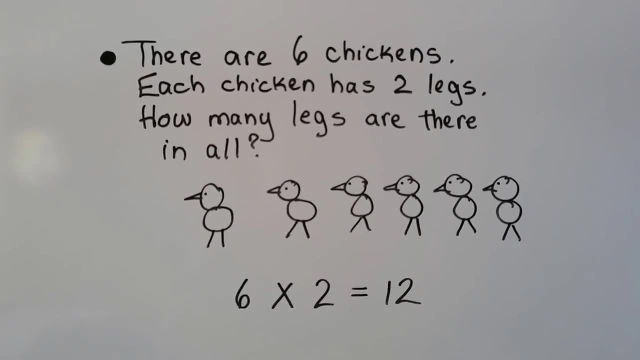 chickens. I usually can draw better than that, but I'm just trying to show you. it's not important how fancy the drawing is. What's important is: did we do a drawing that correctly describes the problem? There's one, two, three, four, five, six chickens. 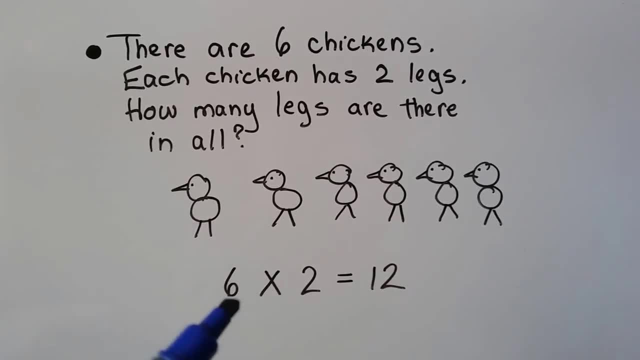 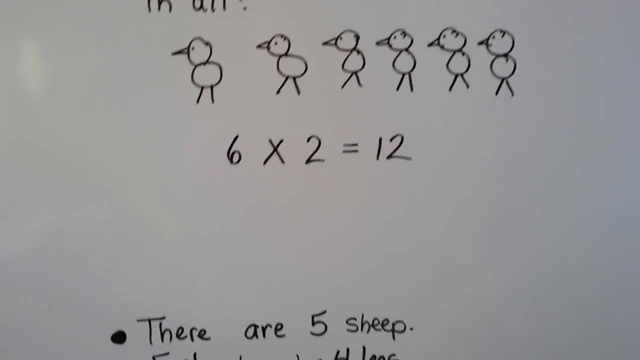 Each of them has two legs. That means we have six times two legs. That equals 12.. See, Don't worry about how fancy your drawing is. all right, There are five sheep. Each sheep has four legs. How many legs are there all together? 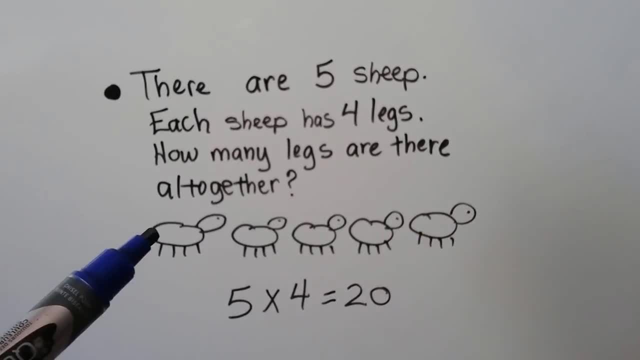 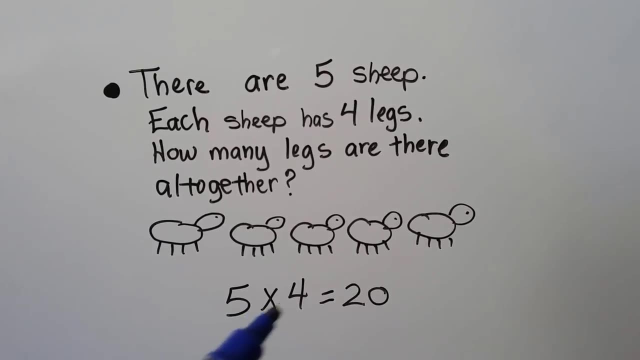 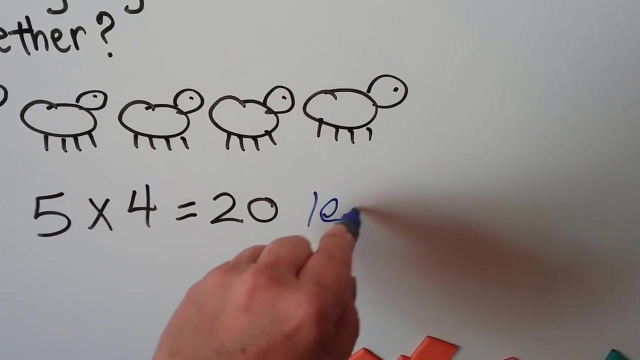 Just draw five little animals and give each one four legs. We have five animals. five sheep times four legs, We have 20.. And that would be 20 legs, wouldn't it? Okay, We need to label our answers, all right. 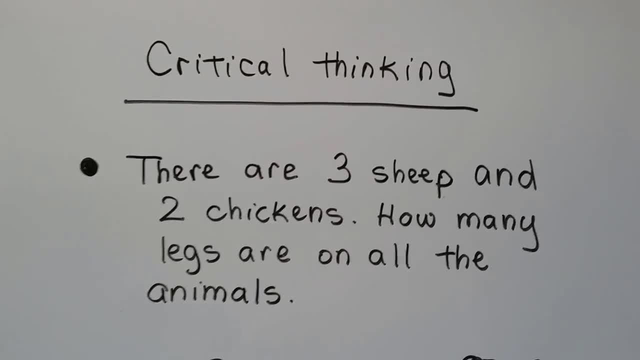 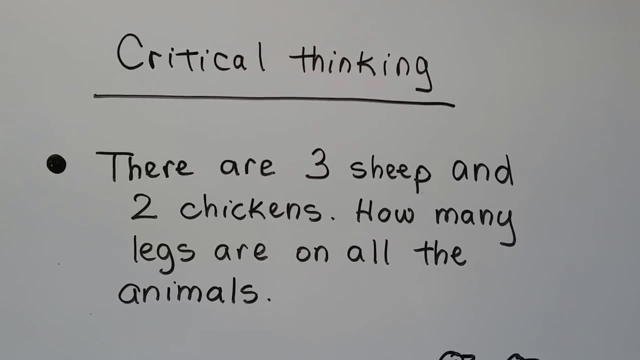 So let's take a look at this one. This is critical thinking. It says there are three sheep and two chickens. How many legs are on all the animals? Well, they have different numbers of legs, don't they? Sheep have four legs and chickens have two legs. 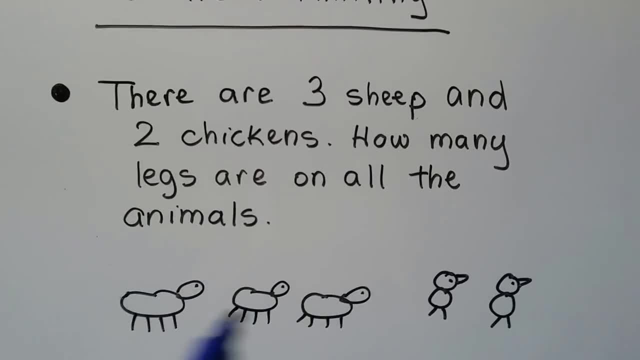 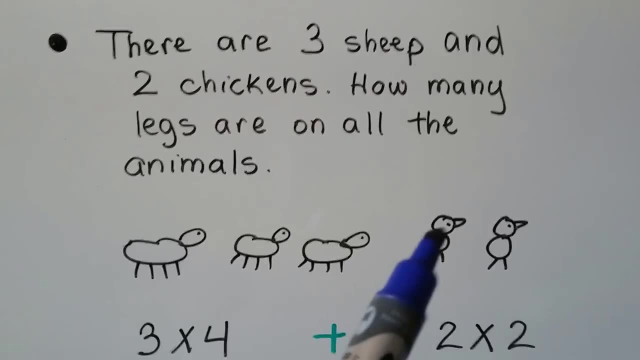 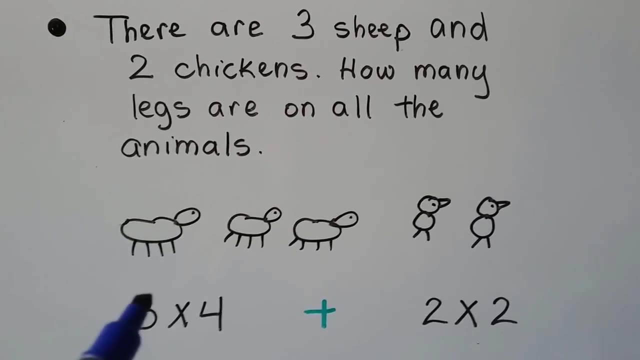 Well, if there's three sheep, we can draw three sheep and we can see that's three times four legs. The two chickens: we can draw two chickens and they each have two legs, so we have two times two. We can answer this: one: find the product. 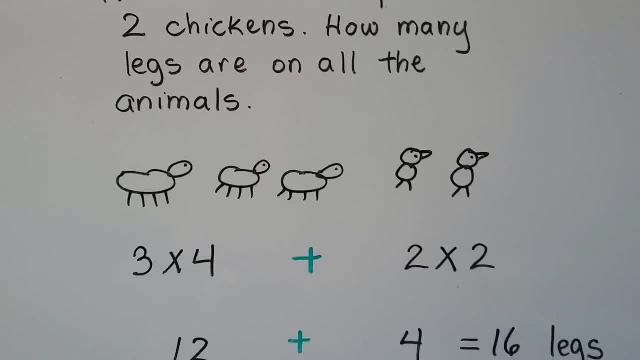 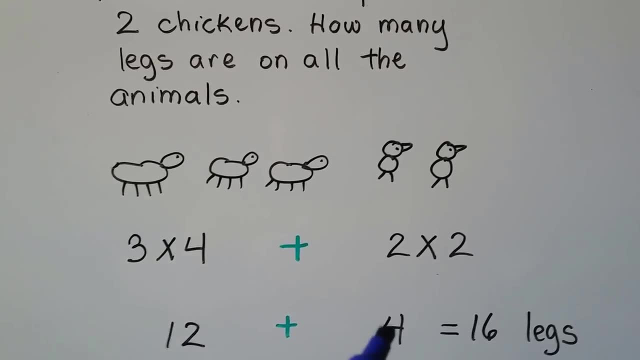 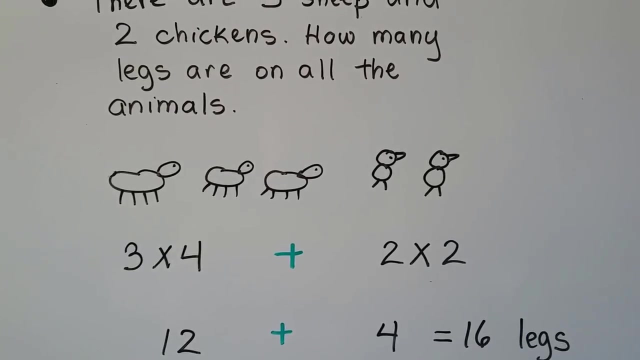 and answer this one and find the product and then add them together. Three times four is 12, and two times two is four, and then we add the 12 plus the four And we get 16 legs. See, And make sure you label that that's the legs, okay.